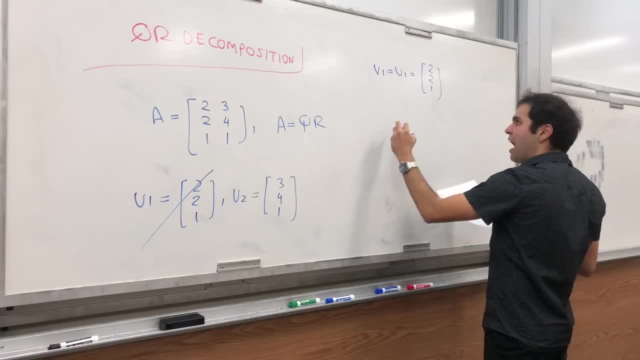 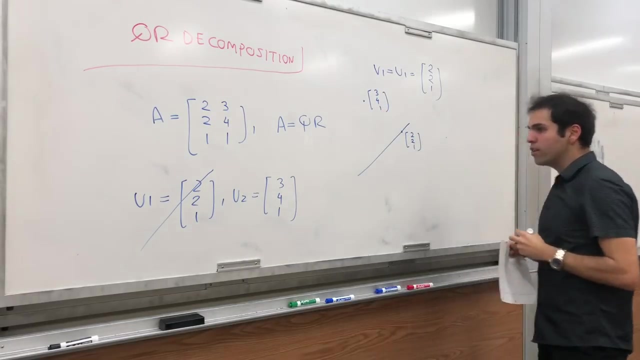 And then what's the situation? You have this vector 2, 2, 1, which spans a line, maybe here, And now you have this other vector 3, 4, 1.. And what you would like to do is so this is U2.. 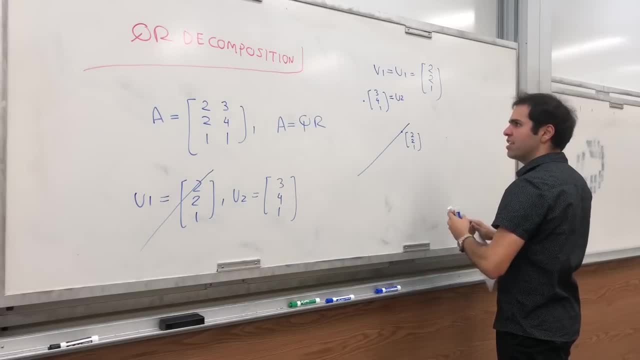 You would like, first of all, to squish this vector on this line. In other words, you would like to calculate the orthogonal projection. So this is U2 hat. And how do you construct U2 hat? So this is V1 here. 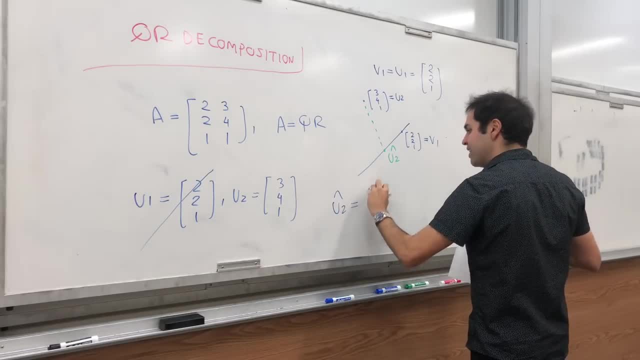 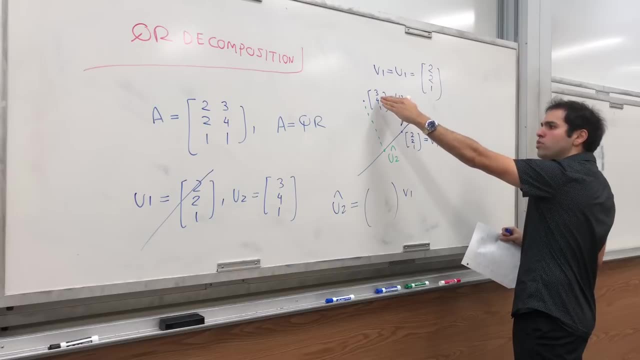 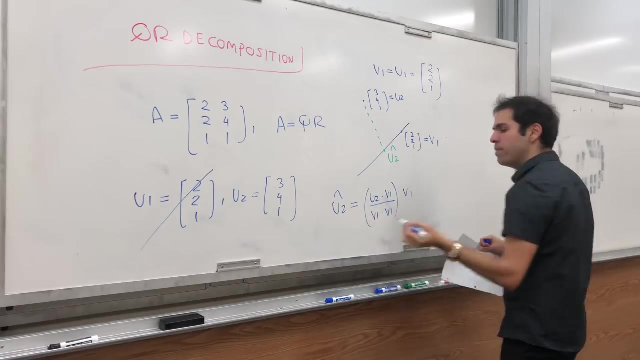 So U2 hat is just, it's a multiple of V1. So something times V1. And to do that you just do U2 dotted with V1. So U2 hugs V1. And then V1 is so happy it hugs itself. 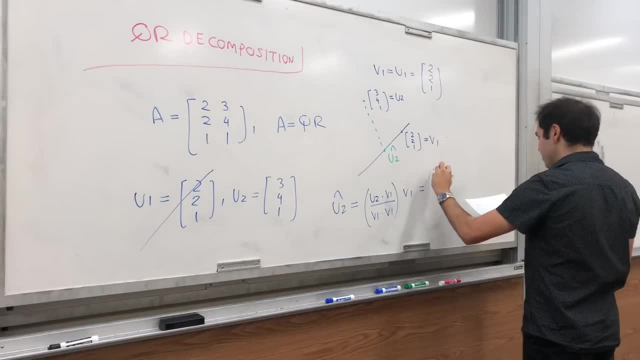 Okay, And in this case, what this becomes, this is, you know, a 3, 4, 1. Dotted with 2, 2, 1.. Over 2, 2, 1. Dotted with 2, 2, 1.. 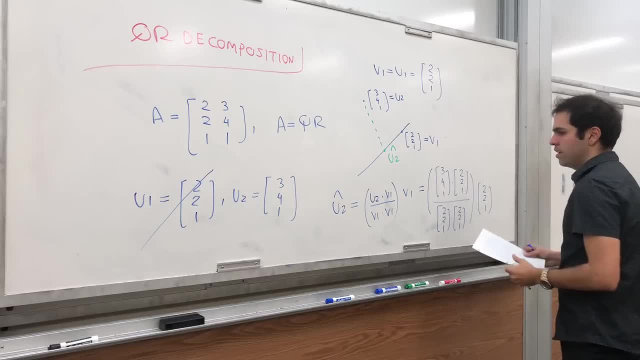 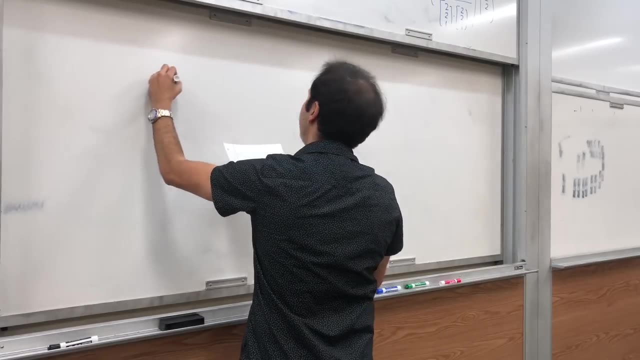 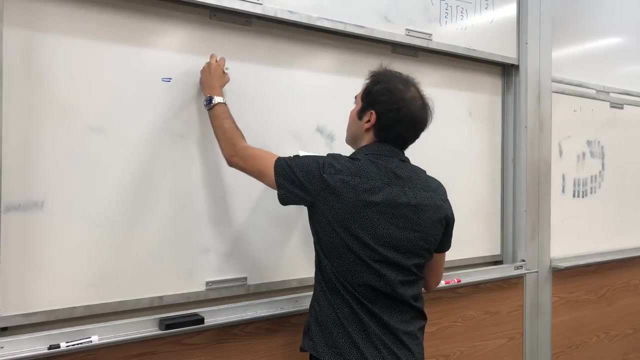 Times 2, 2, 1.. And again it has to be a multiple of 2, 2, 1.. And if you calculate that, I believe you get 15 ninths. Let me see 6 plus 8, 14 plus 1, which is 15.. 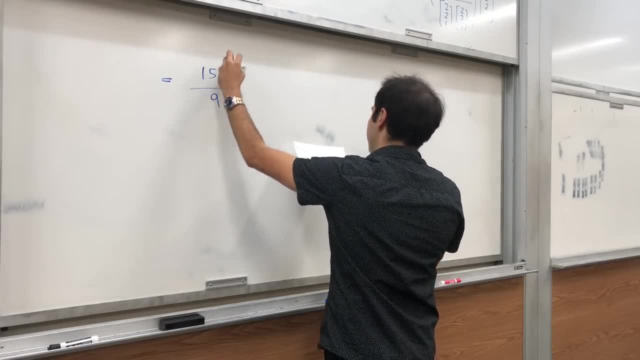 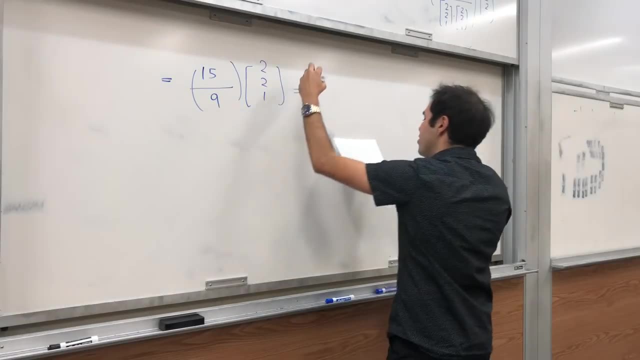 And 4 plus 4 plus 1, which is 9.. So yes, 15 ninths times 2, 2, 1.. 15 ninths is 5 thirds. So in the end you get 10 thirds, 10 thirds, 5 thirds. 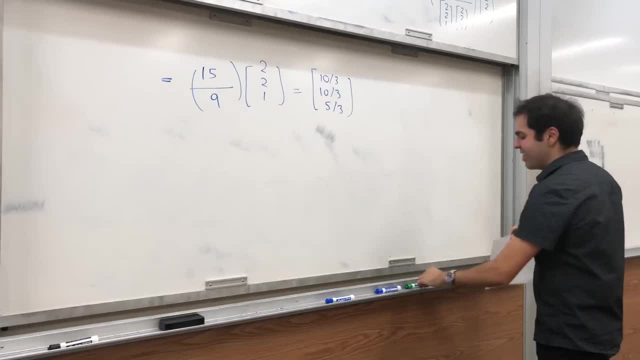 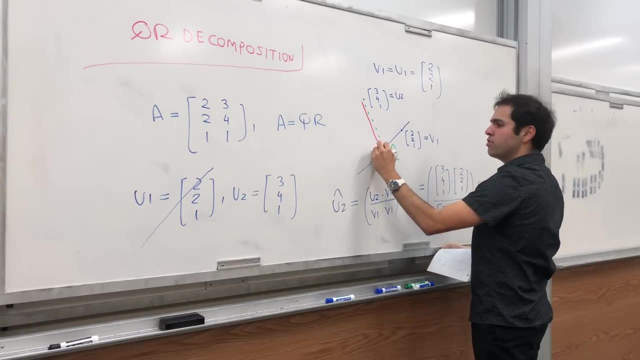 And again, careful, do not rescale this, Otherwise you get a wrong answer. And then how do you do this? And then how do you define your V2? It's simply a vector perpendicular to V1. Which, in this case, it's U2 minus U2 half. 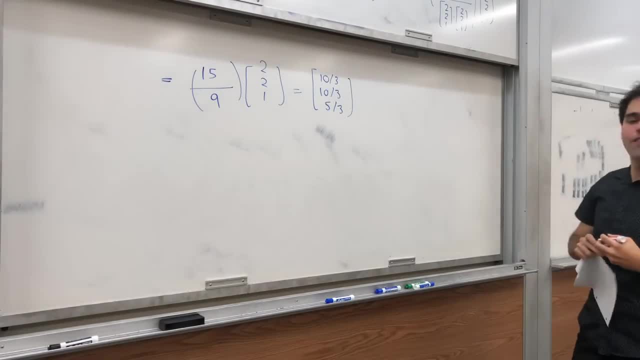 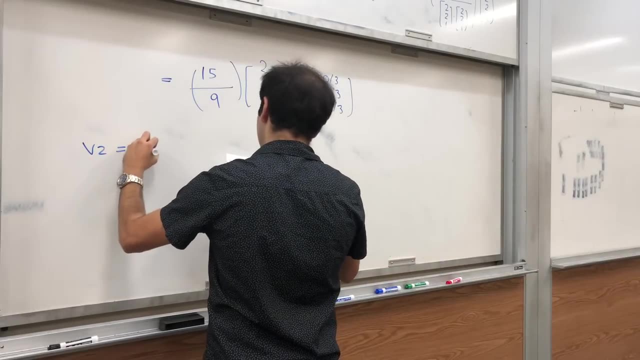 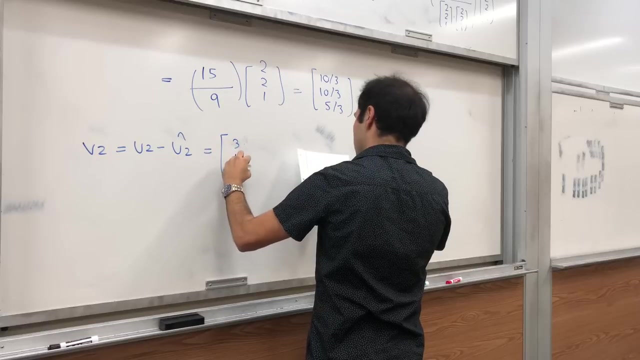 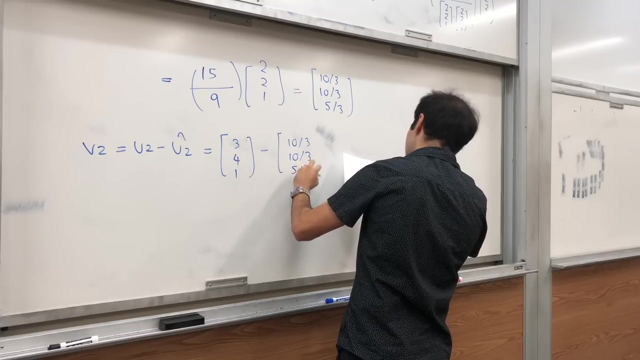 And that was the whole point of orthogonal projections- is to find a vector perpendicular to another one. So V2 is then U2 minus U2 half, And that's 3, 4, 1. Minus 10 thirds, 10 thirds 5 thirds. 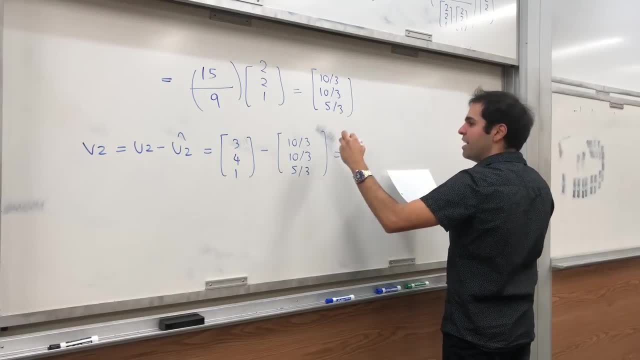 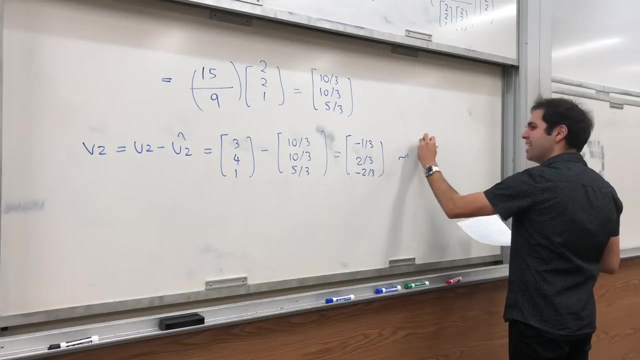 And that's just 9 thirds minus 10 thirds. So minus 1 third, 2 thirds And then minus 1 third. I saw minus 2 thirds. You could rescale it, So it's totally fine to say minus 1, 2,, minus 2.. 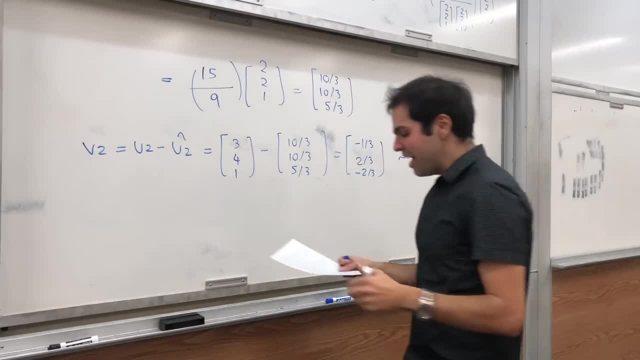 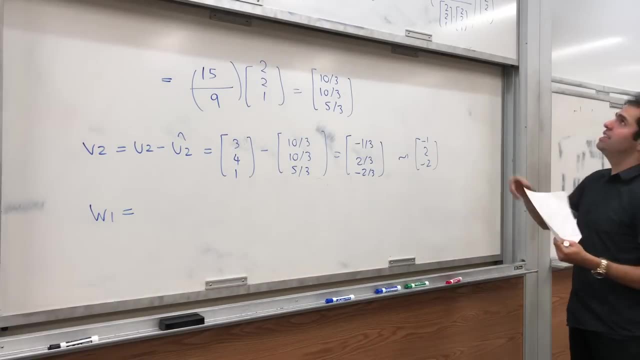 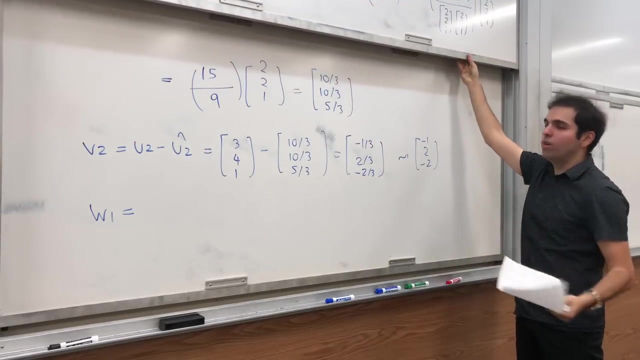 But you'll see in a second why this is useful Then. so this gives you an orthogonal basis, So you can indeed check that if you do V1, so 2, 2, 1, dotted with minus 1, 2, minus 2,. 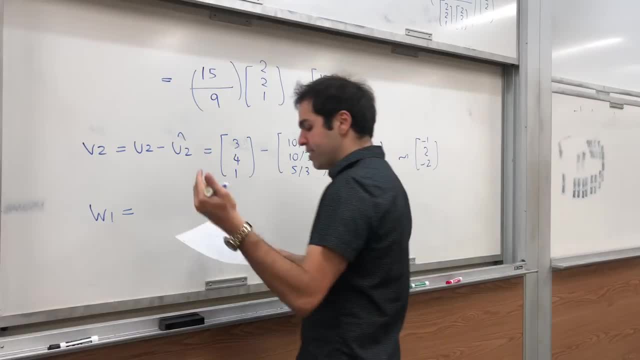 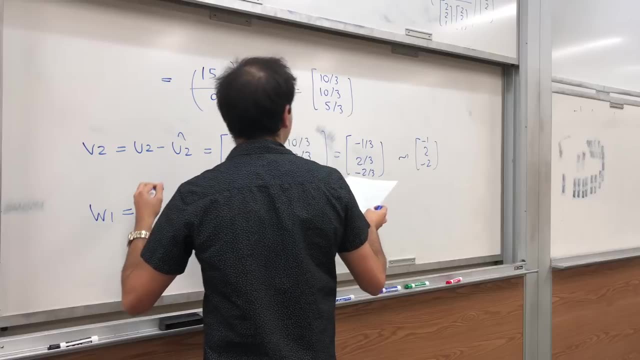 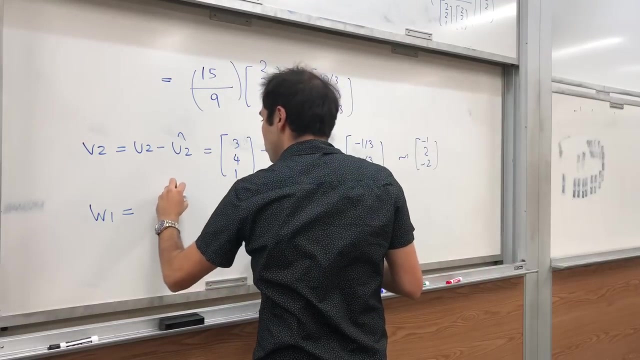 you get 0.. And lastly, since you want a matrix with orthonormal columns, you just get- I'll talk in a second about that, So I just realized something. Then you just get. so 2,, 2,, 1,. 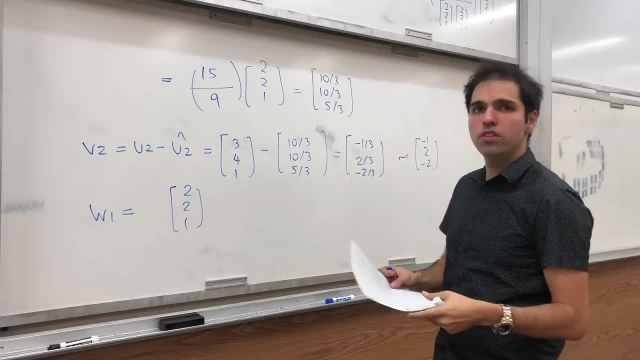 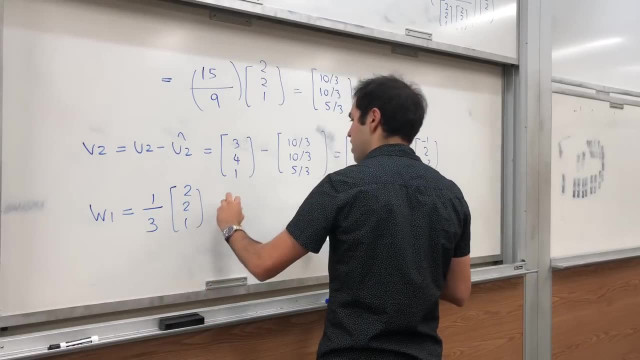 the length of 2,, 2, 1,. it's square root of 2 squared plus 2 squared plus 1.. So square root of 9, which is 3.. And we get 2 thirds, 2 thirds and 1 third. 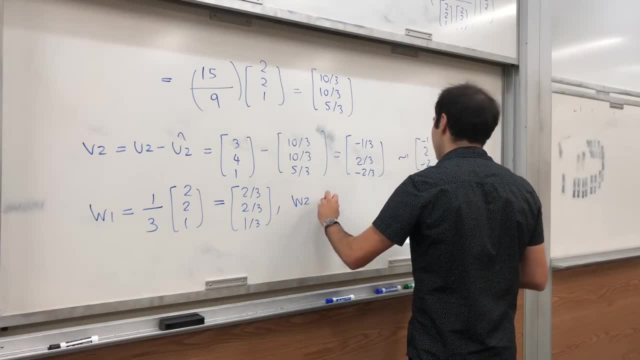 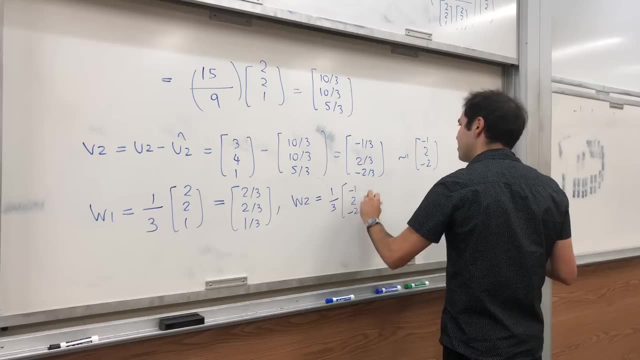 And for the second one again, the length of this is 9,, so 1 third times minus 1,, 2 minus 2.. And you would feel a bit silly because you would get minus 1 third, 2 thirds. 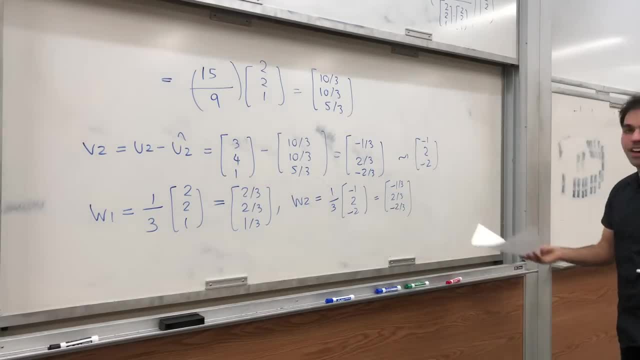 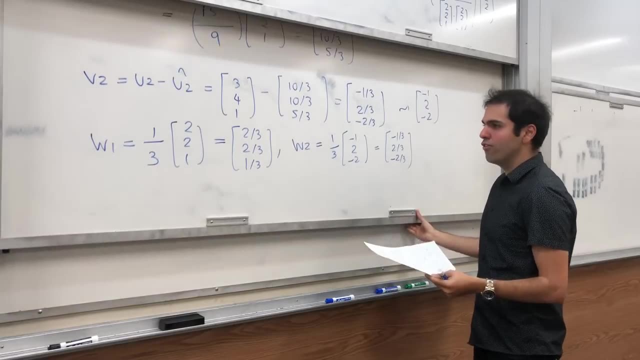 and minus 2 thirds Ta-da. Okay, so this is, you know, your orthonormal basis. And then, of course, the question is: how do you find your matrix Q? Well, you just put both of them together. 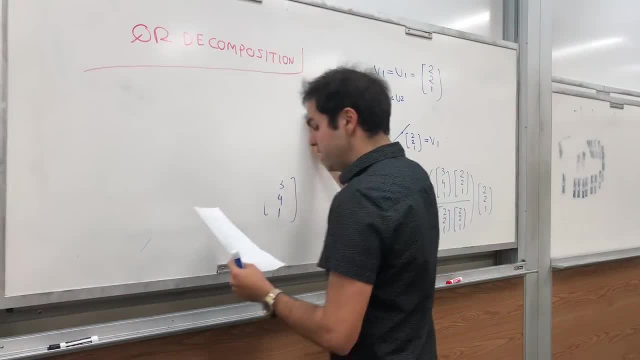 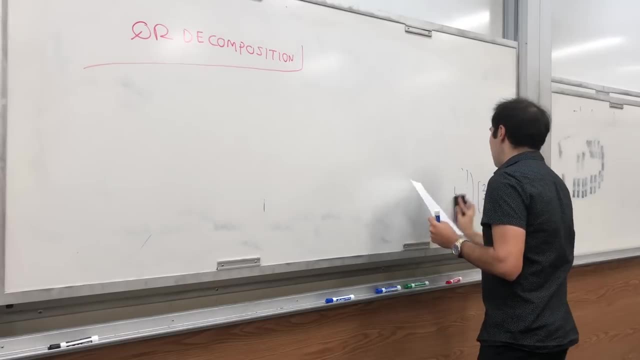 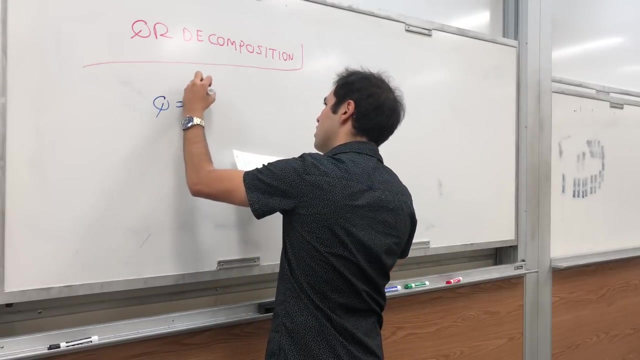 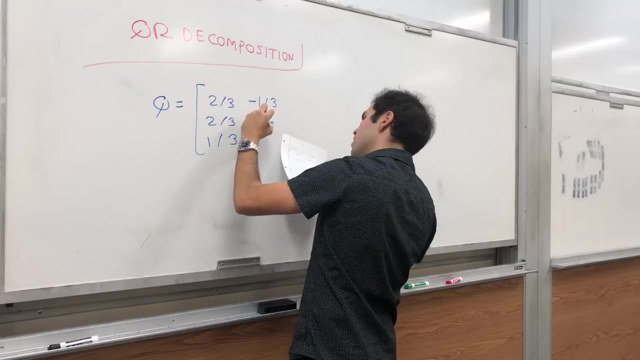 So indeed you get, A is Q, or well, at least Q is the matrix with orthonormal columns. So Q is 2 thirds, 2 thirds, 1 third and minus 1 third, 2 thirds minus 2 thirds. 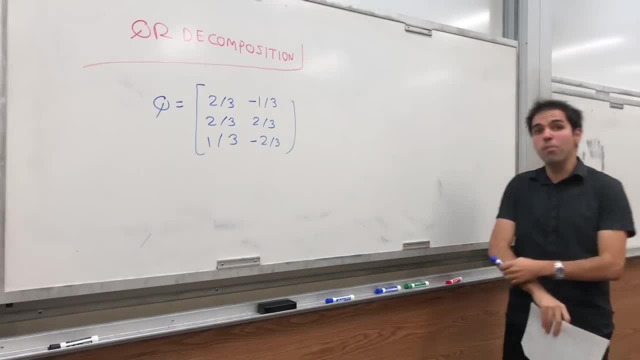 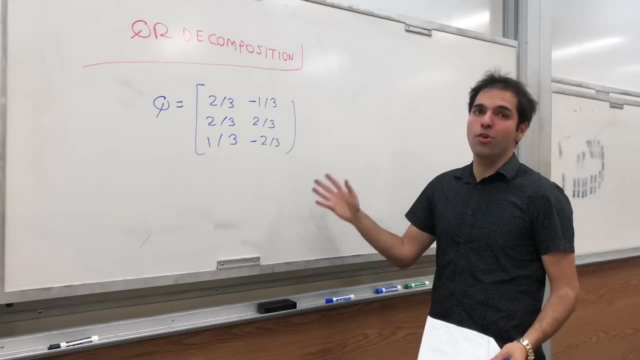 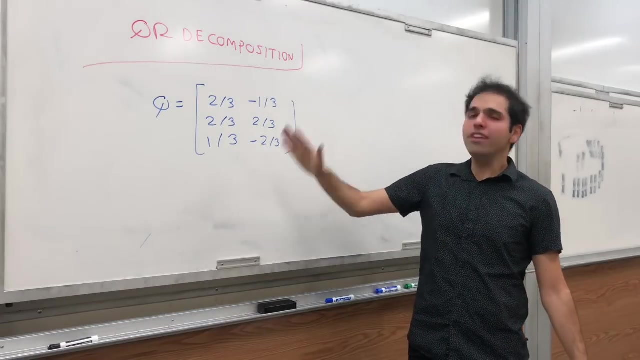 All right, I just realized something. So many books define an orthogonal matrix to be a square matrix whose columns are orthonormal. For me, I think it's a silly convention. I would still call this an orthogonal matrix, But really what it is, it's a, you know, rectangular matrix. 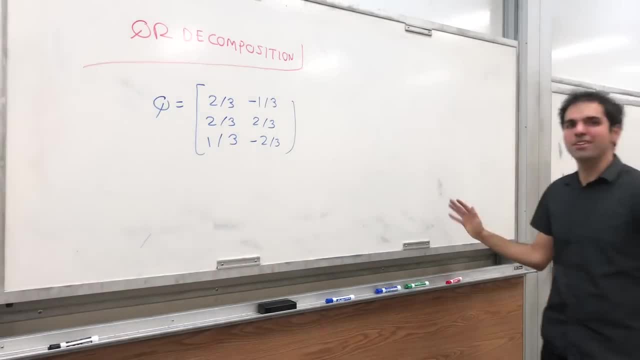 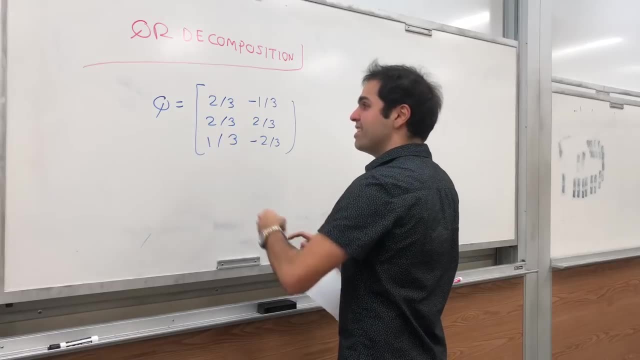 whose columns are orthonormal. So if you're picky about this, okay, It's not an orthogonal matrix, but come on, Okay. So this is Q, And the question is: how can we find R? It's actually a very cute calculation. 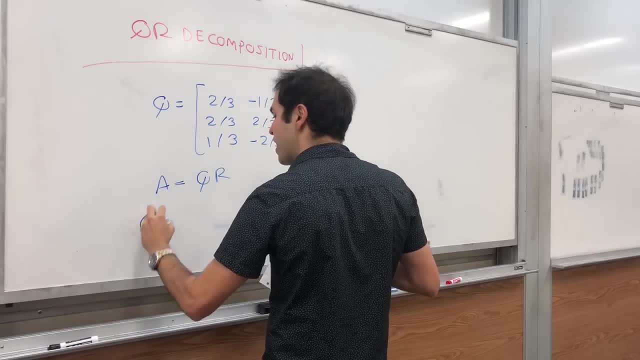 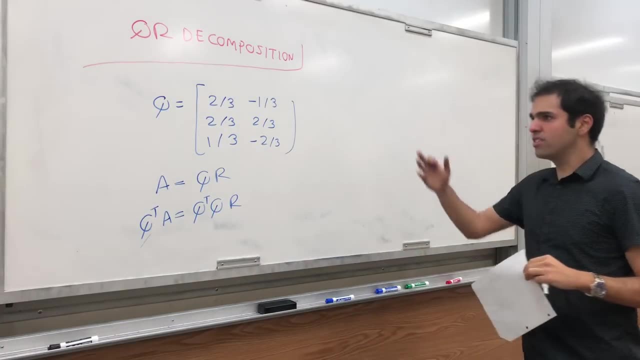 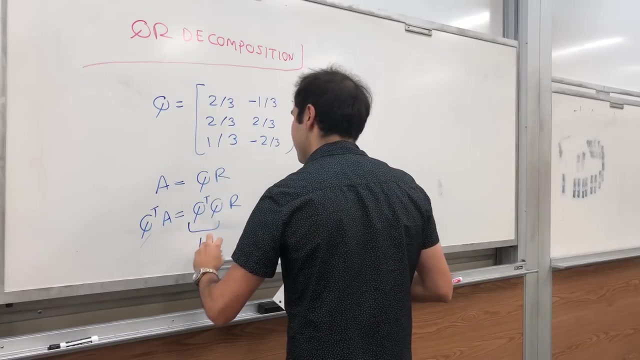 So if A is QR, then calculate Q transpose A, That is, Q transpose QR, And since Q has orthonormal columns, it turns out Q transpose Q is the identity. So we just get IR. You're on. Okay, That's R. 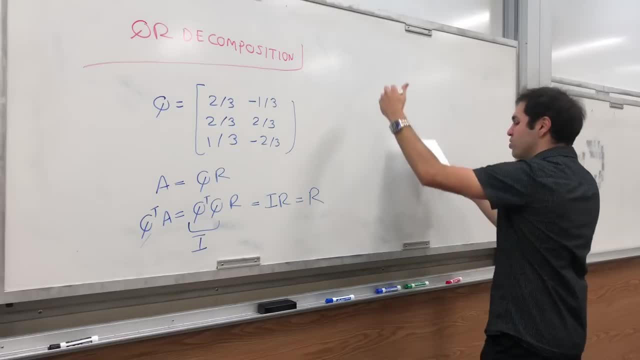 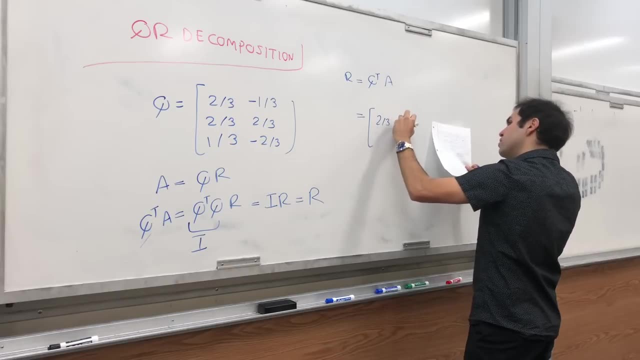 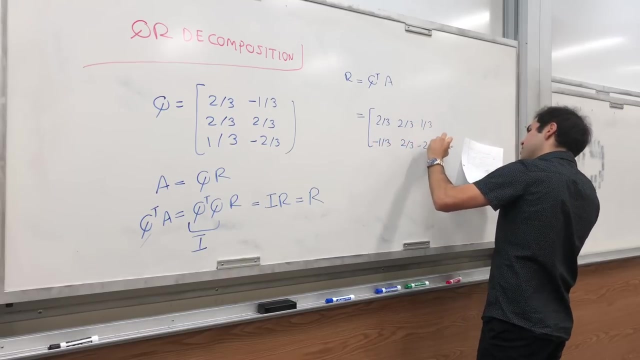 So, in other words, reversing this, you get R is just Q transpose A, which in this case it's 2 thirds, 2 thirds, 1 third minus 1 third, 2 thirds minus 2 thirds times 2, 2, 1, 3, 4, 1.. 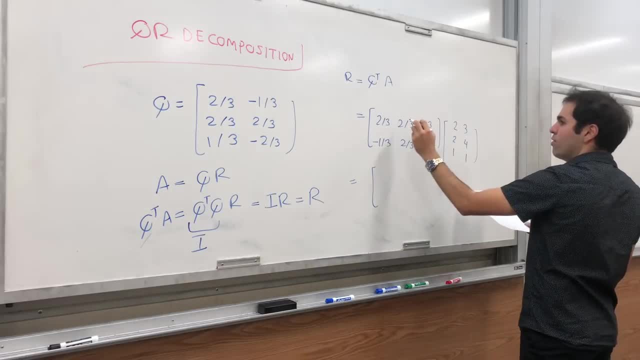 Okay, And then I believe you get so 4 plus 4.. So 8 plus 1.. So 9 thirds, which is 3.. And then 6 plus 8.. So 14 plus 1.. 15 over 3, 5.. 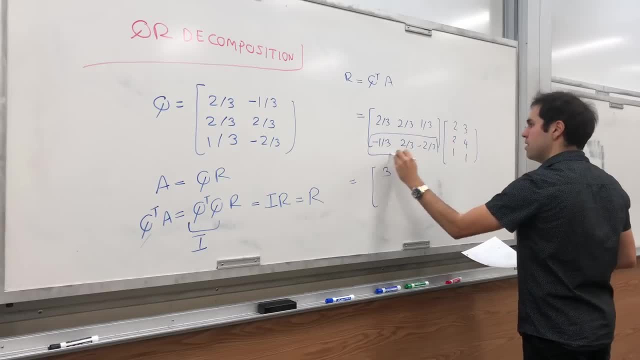 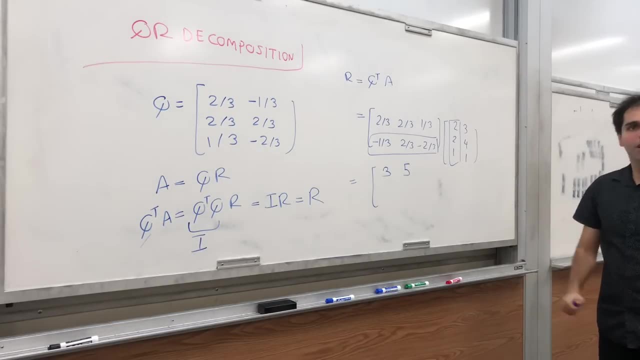 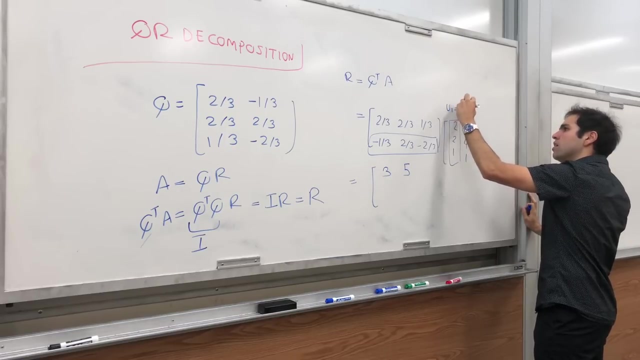 And here comes the interesting thing: If you dot those two vectors, you will get 0,, which is surprising. but you shouldn't be surprised Because, remember, this was the first vector of your Gram-Schmidt process. So this was, I guess, U1, which is V1, right? 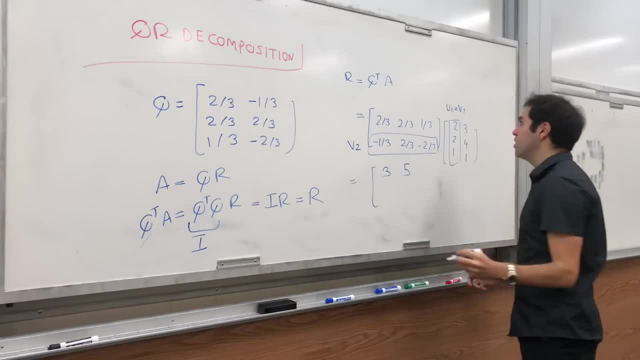 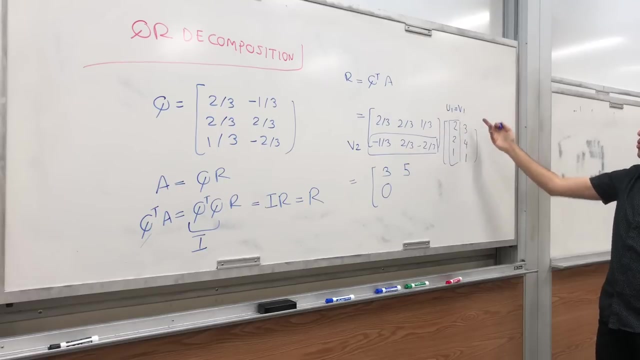 And this is your vector U2.. I'm sorry, V2.. So by definition, if you dot those two vectors, you should get 0. So that's why it's 0. And for higher matrices. so it won't really be V2 dotted. 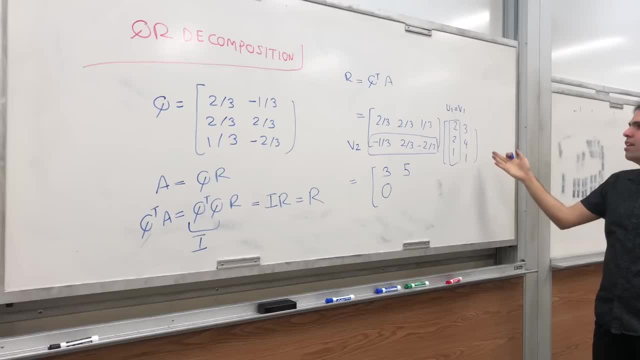 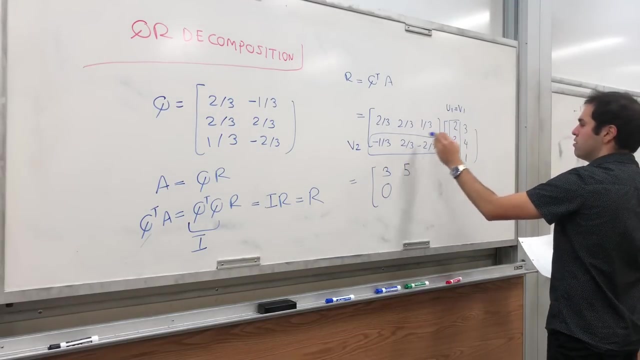 with V1, but probably V2 dotted with, or V3 dotted with some vector in the span of V1 and V2.. So this is why, in general, R will be an upper triangular matrix, And then, if you do the last one, you get minus 3.. 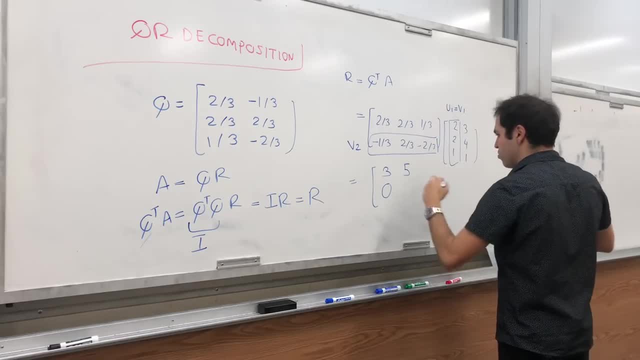 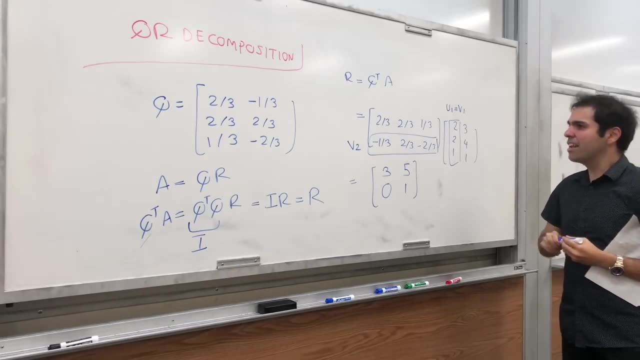 So 5 minus 2,, so 3,, which is 1.. And so in other words here, yes, R is an upper triangular matrix, And for me that's enough. But it turns out you can even tweak this by getting just positive entries on the diagonal. 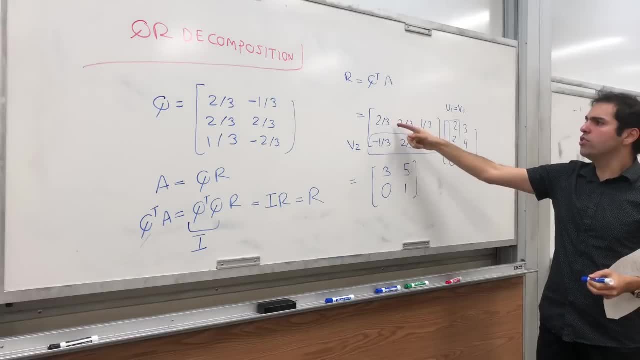 And that's basically by changing your vectors by minus a vector. So if you get a negative entry, just change one of those columns by minus and then it should be fine. OK, All right, great. So we found Q, We found R. 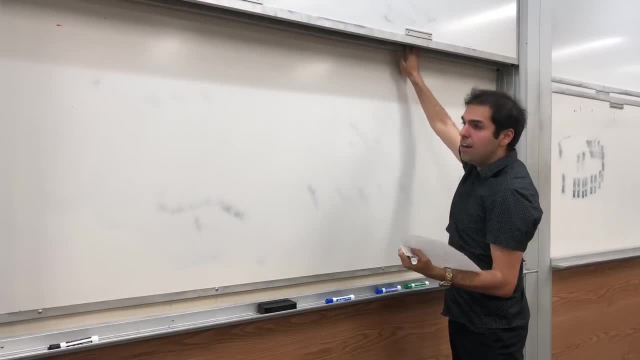 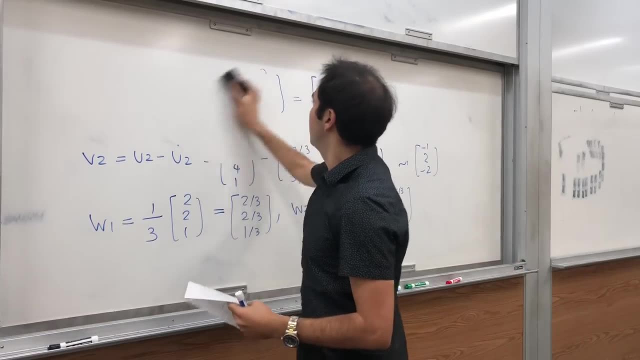 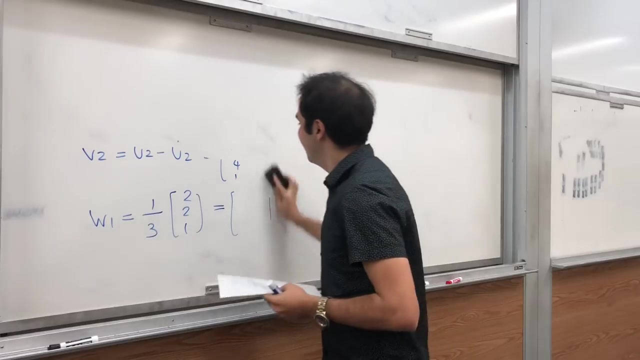 And you can check that A is QR. But now let me tell you why it's so useful to find in practice, Because there must be a reason why I tell you about this. This has to be useful in some sense. It's useful if you want to find least-square solutions. 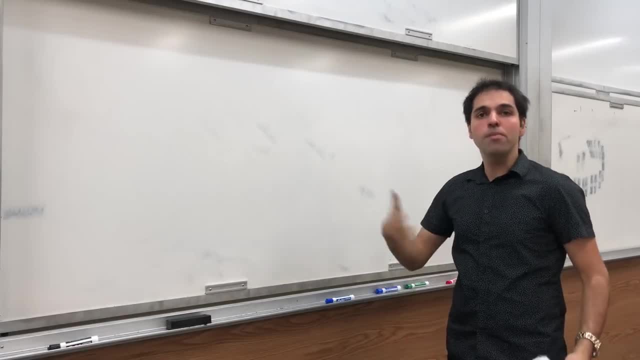 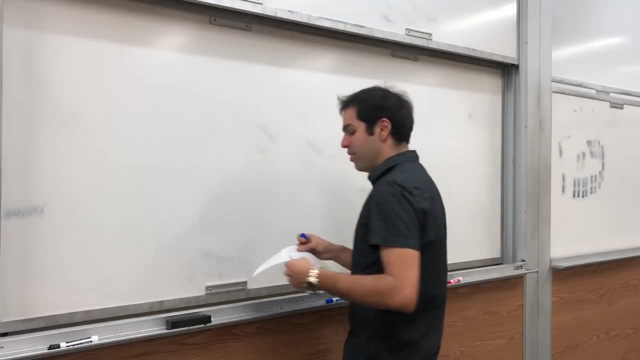 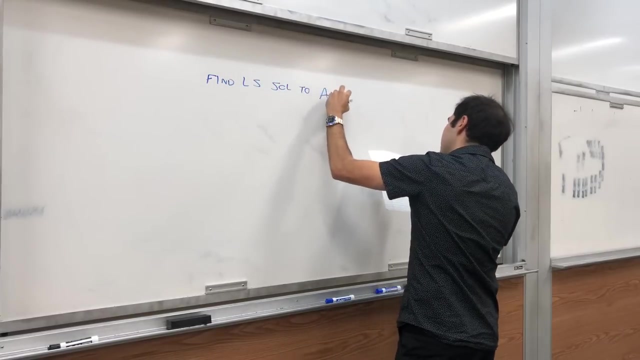 And remember least-square solutions. what's happening is some equations have no solutions but you still want to have sort of the best non-solution. So suppose you find a least-square solution to AX equals 7,, 3,, 1,. 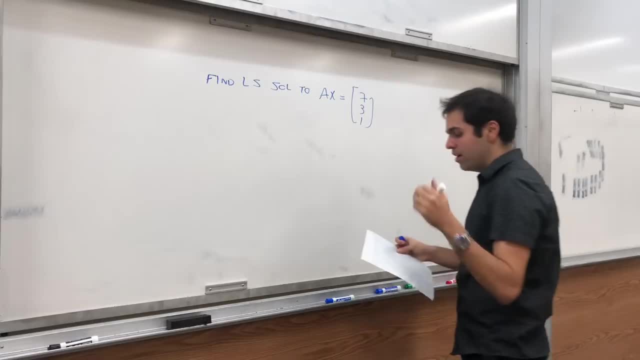 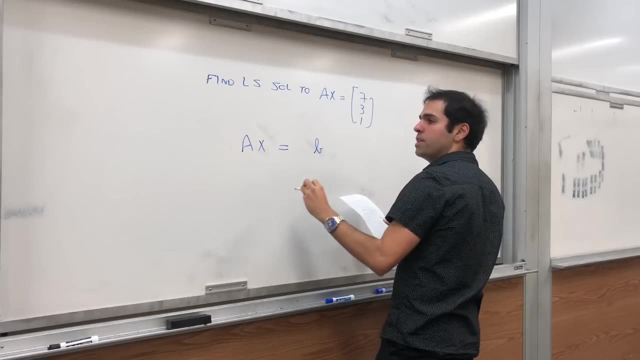 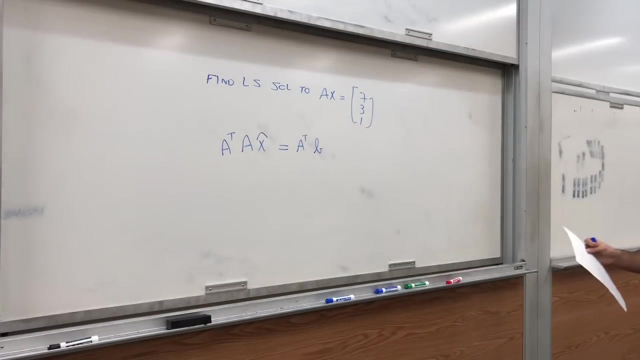 where A was the matrix as before. Then remember how to find least-square solutions. You just do: you take AX equals B and you multiply by A, transpose. That gives you your solution of ATAX. hat equals to ATB and X, hat is the least-square solution. 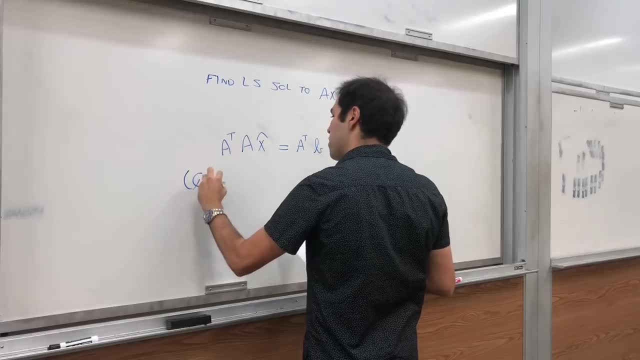 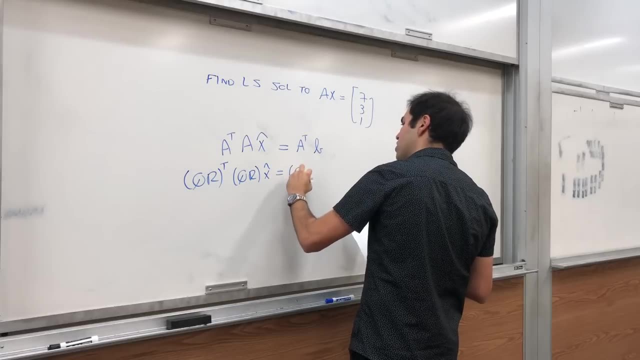 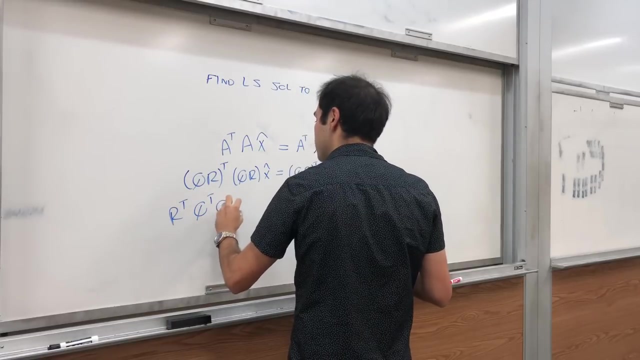 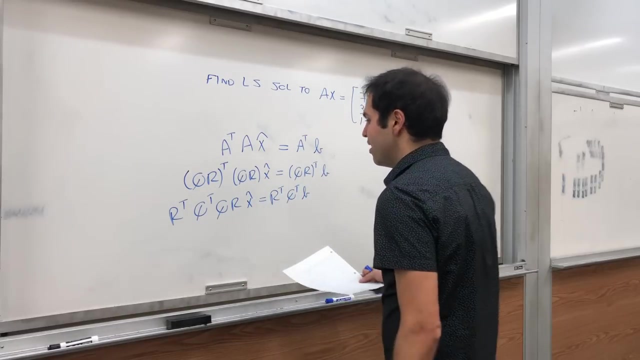 But now suppose A is QR, Then we get QR transpose QRX hat equals QR transpose B. And then R transpose Q transpose QRX hat. it's R transpose, Q transpose B. Well, look, Q transpose Q. by definition, that's just the identity. 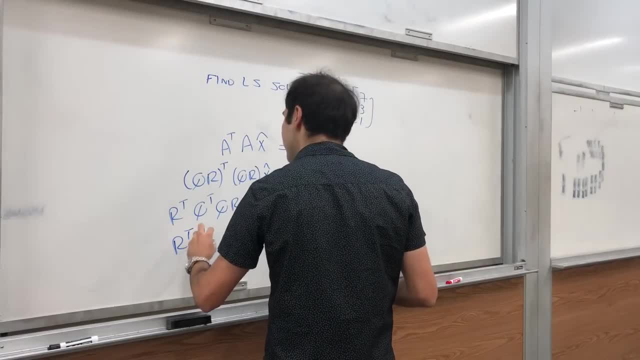 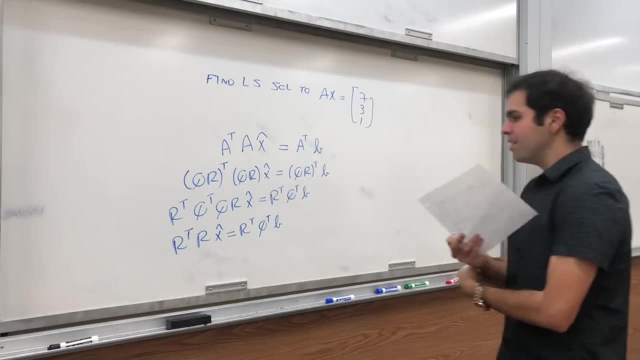 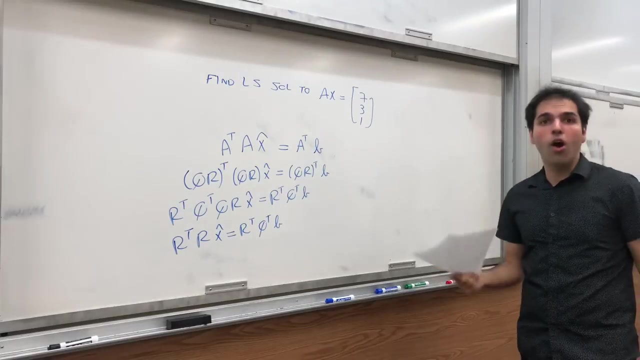 because Q has orthonormal columns, So we get R transpose, RX hat equals R transpose, Q transpose B. And now, well, you would like to cancel out R transpose and the thing is it's not always possible. So it's not always possible that R is actually invertible. 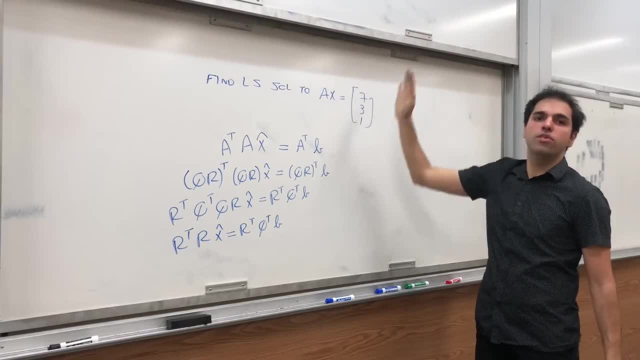 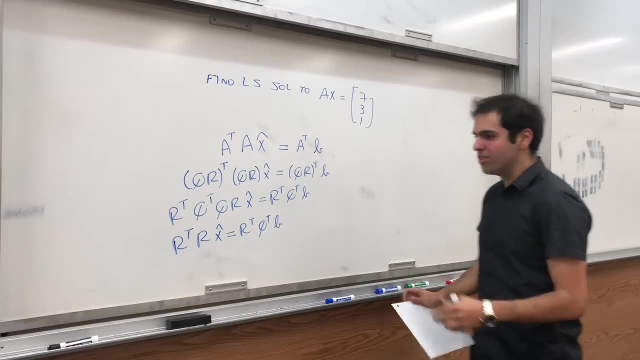 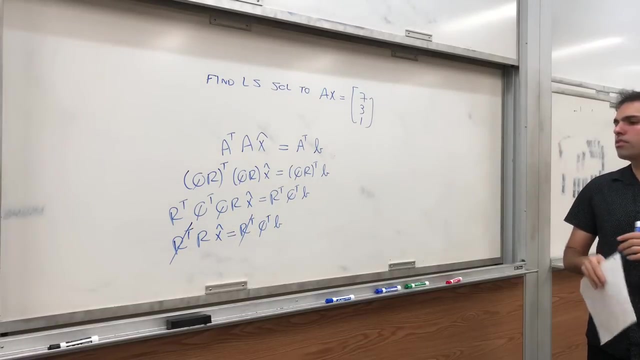 And that would basically happen if there's no least-square solution. So 99% of the time, R will actually be invertible, So in that case you can actually cancel it out. So and the thing is basically what we would need to do. 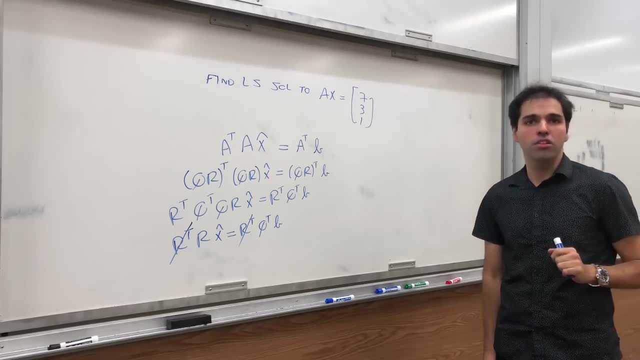 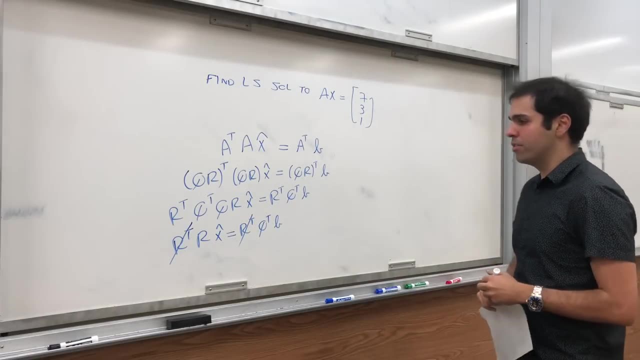 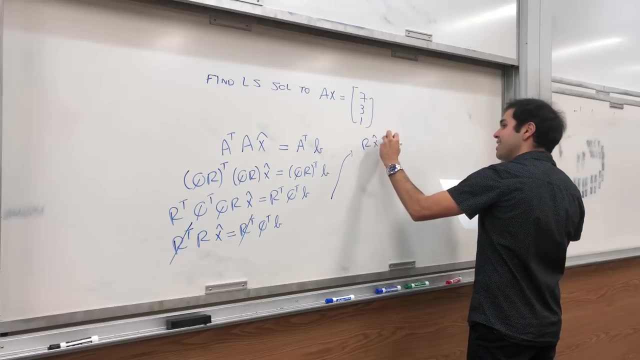 is having A having N linearly independent columns. So the columns are A If they're linearly independent, turns out that R is in fact invertible. So and then what you get is in the easier equation: RX hat equals Q, transpose B. 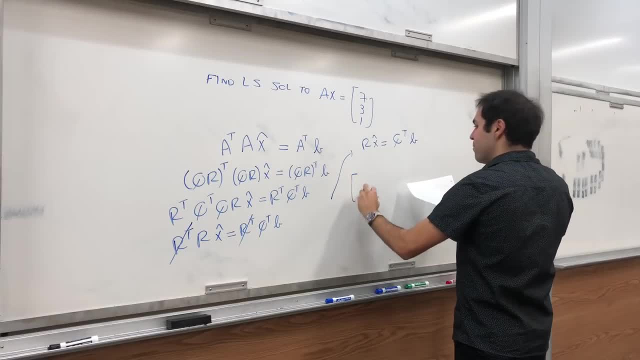 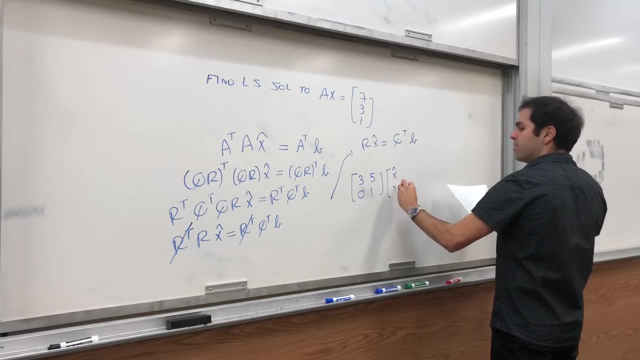 And let me show you why it's such an easy equation: Because R is upper triangular, So you have to solve 3,, 5, 0, 1, let's call X hat by abuse of notation. let's call the variables X hat and Y hat. 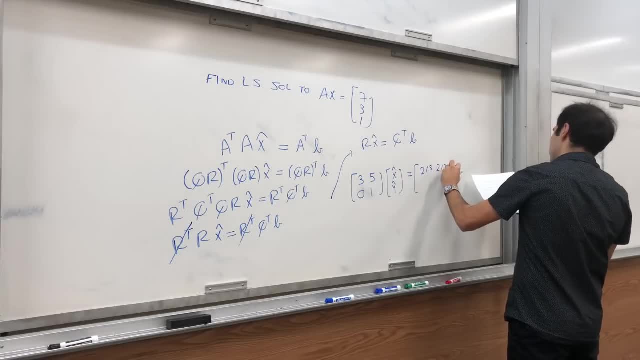 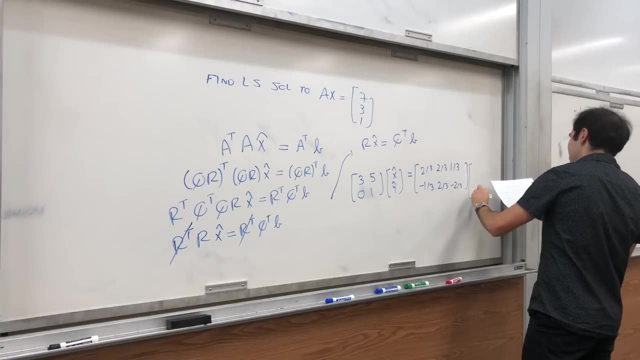 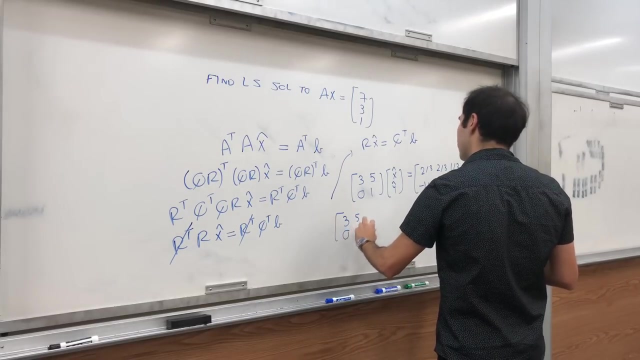 equals 2 thirds, 2 thirds, 1 third minus 1 third, 2 thirds minus 2 thirds: 7, 3, 1.. And if you do that, you get 3, 5, 0, 1,.